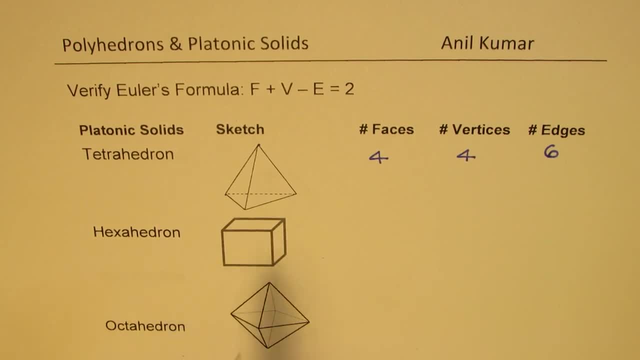 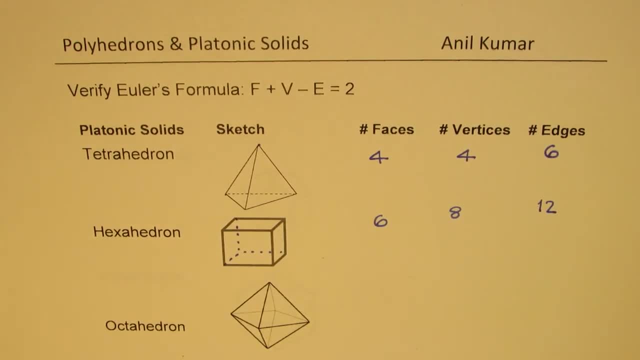 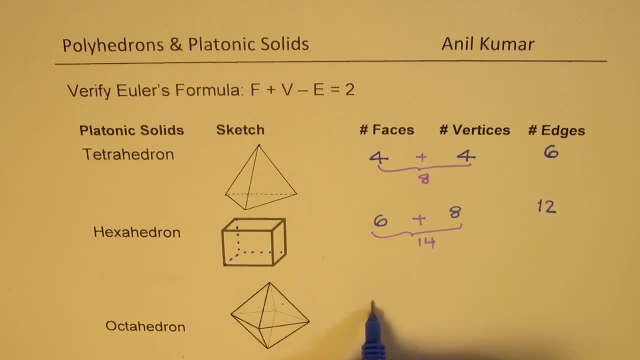 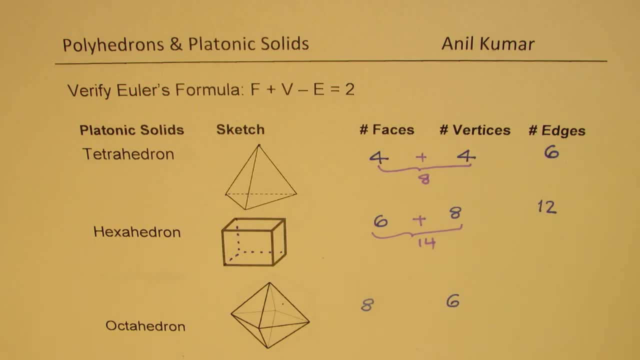 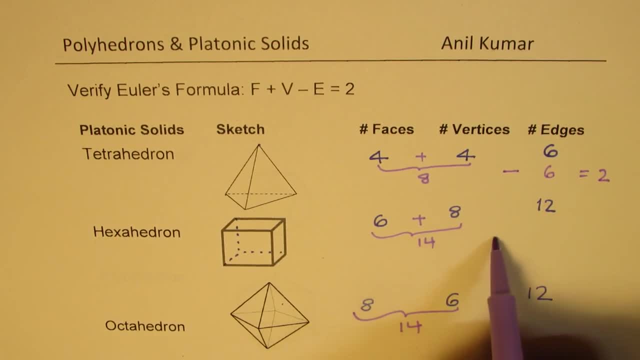 the number 6, we do get 2, right? In this case, if I take away 12, we do get 2.. And in this case also, if I take away 12, I do get 2.. So all three of them, we have verified that the Euclid's 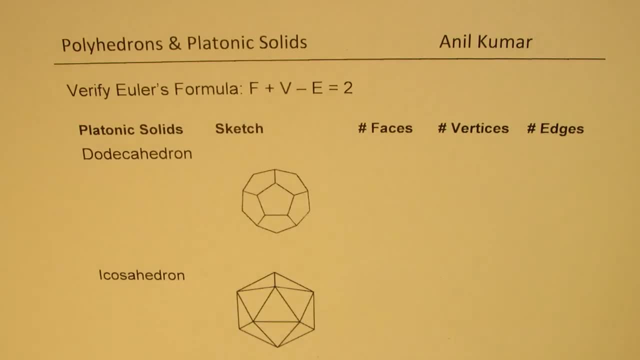 formula works for them. Now let's look into the more complicated platonic solids. Now here, dodecyhedron, we have pentagonal faces right, So you can see the top portion, So which we have 1,, 2,, 3,, 4,, 5,, 6, and we have 6 on the other side, right, So that makes it 12 faces. 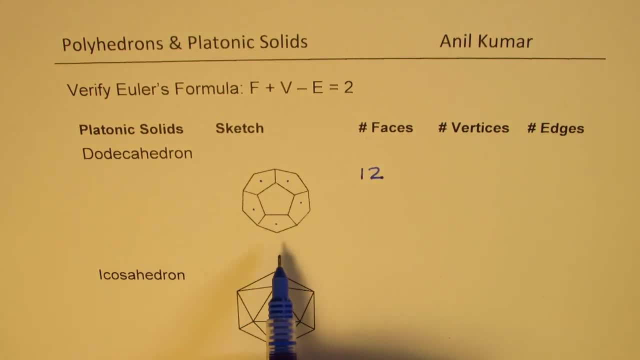 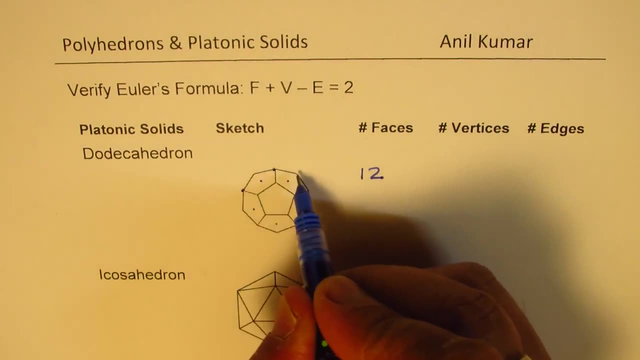 correct 12 faces Now as far as the vertices are concerned. so let's count the vertices here one by one. So we have 1, 2, sorry, I missed this one. So it's a pentagon, right. So 1,, 2,, 3, 4,, 5,, 6,, 7,, 8,, 9, 10.. Now, this is common to both the edges. 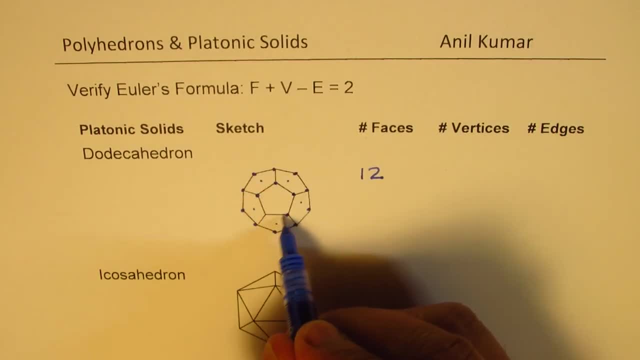 right: 11,, 12,, 13,, 14,, 15.. And then again 16,, 17,, 18,, 19,, 20 on the backside, correct? Yes, So we do have 20 vertices As far the edges are concerned. so these edges double up. So 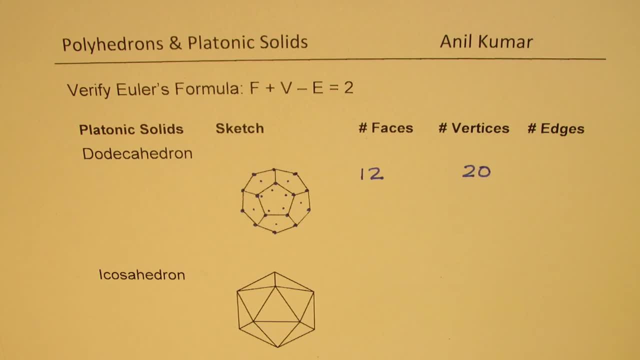 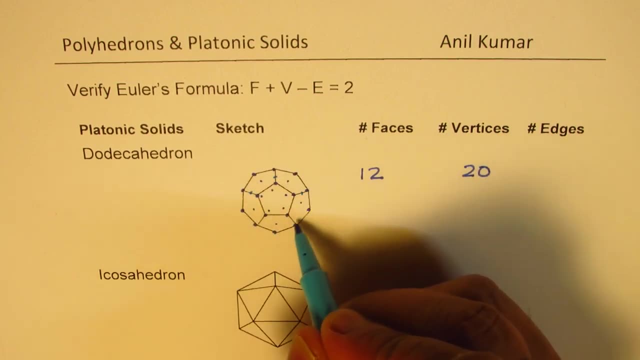 let's count these edges one by one. Let me take a different ink now. So the edges. So we have 1, 2,, 3, 4, 5, 6,, 7,, 8,, 9,, 10.. And 10, on the other side, makes it 20.. 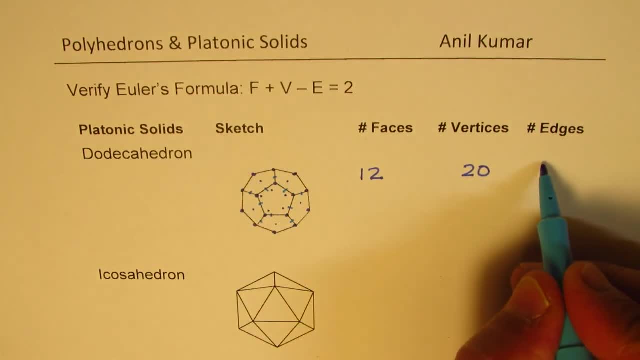 And then we have 10 of these right. So that makes it 30 edges. Do you see that? So we have 30 edges. Now, if I combine faces and vertices, I do get 32.. And 32, take away 30 again gives us 2.. 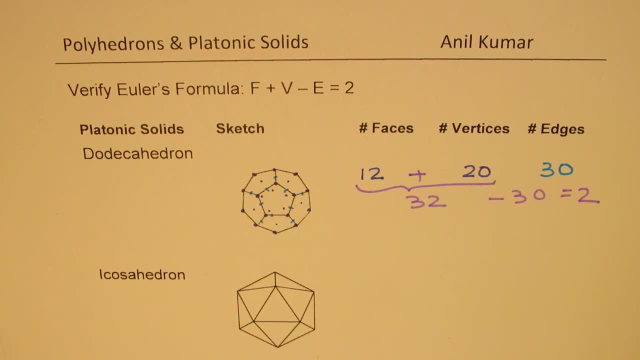 So the Euler's formula is verified here again, correct. Now let's look into icosahedron. Now here we have triangular, So we have triangular faces. As you can see very clearly, we have five faces joining at a point. 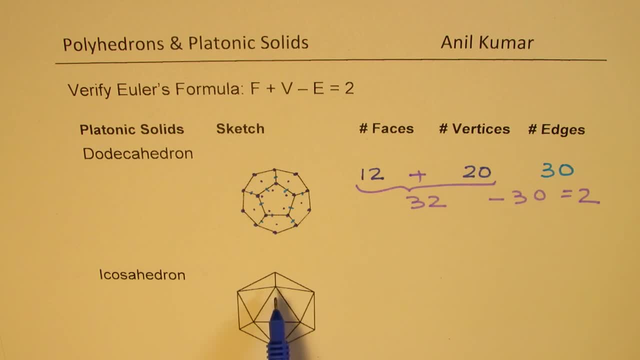 correct. Let's count the number of faces in this case. How many faces do we have? So now, 1, 2,, 3, 4,, 5, 6,, 7,, 8,, 9,, 10, and 10 on the other side. correct, So we have 20 as the name. 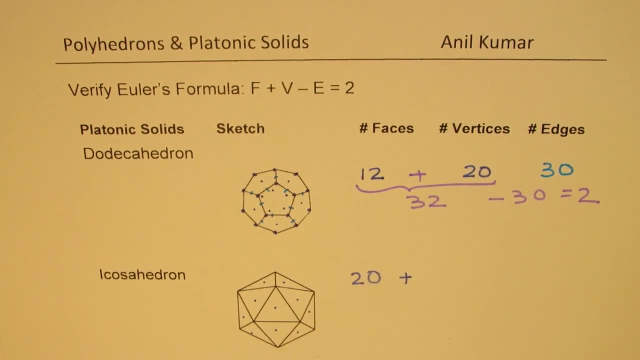 suggests. Now let's count the vertices right Now. these vertices are common right And which develop, are right there in the center. So which is 1,, 2,, 3, right, So these three double ups. 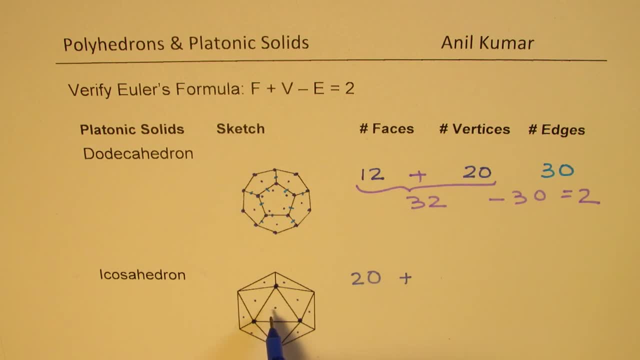 we'll count this 3 and 3 as 6, correct. So we have six vertices right there, And then 7,, 8,, 9,, 10, 11, 12, so we have total of 12 vertices. now let's count the edges. so we know these edges. 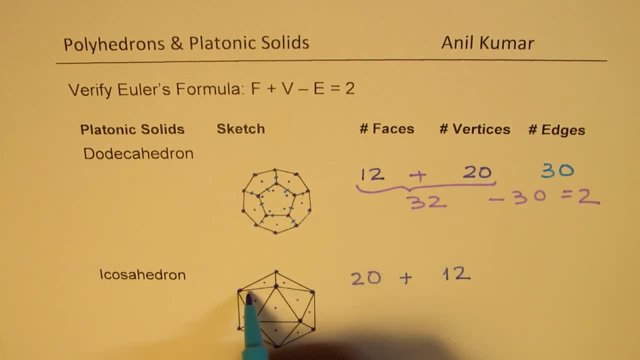 are common to both the outside edges. let's count the inside edges, so we have one: 2, 3, 4, 5, 6, 7, 8, 9, 10, 11, 12. 12 times 2 is 24, and then 25, 26, 27, 28, 29, 30, so we have 30 of these.